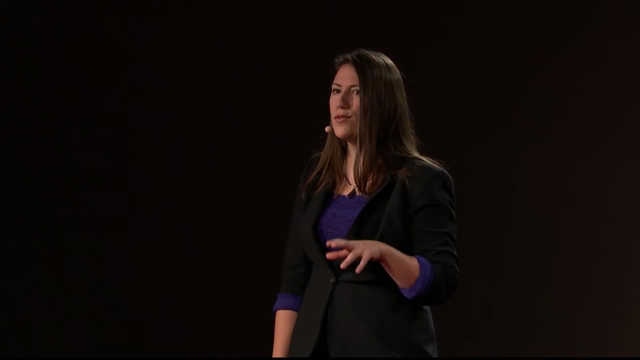 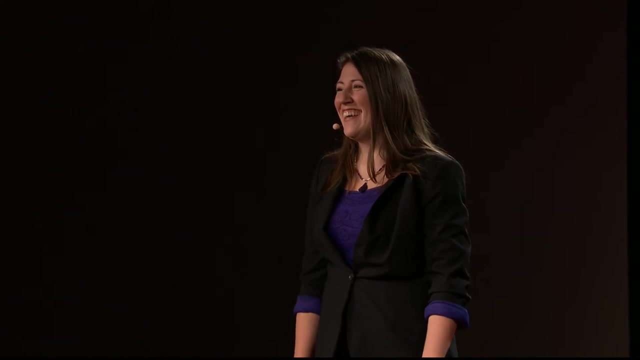 acting school, I switched over to directing because I ran into a few too many situations where a non-native director turned to an all-native cast and said, hey, sing that Indian song, then stared at us waiting. We didn't all magically know the same. 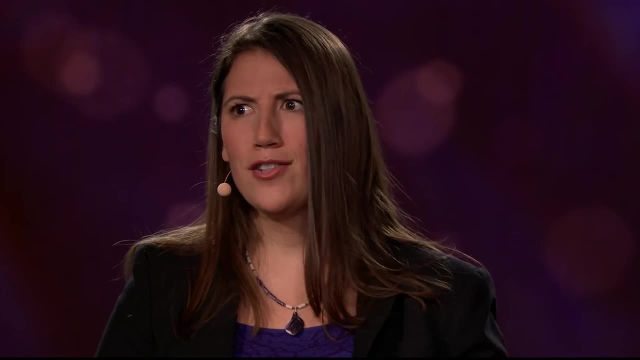 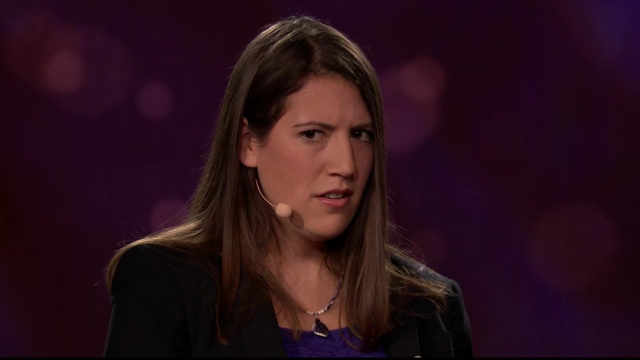 song. We weren't even from the same tribe or culture, yet we were constantly being lumped together into a very finite understanding of what it is to be native Little secret: It's not something that can be checked in a box- One of the most beautiful things about 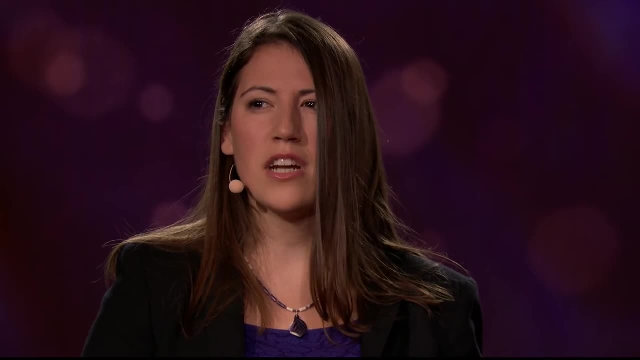 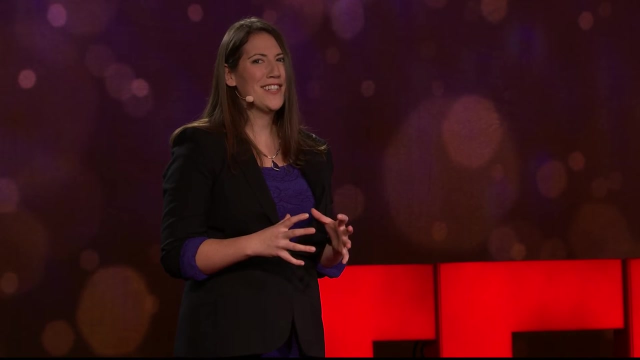 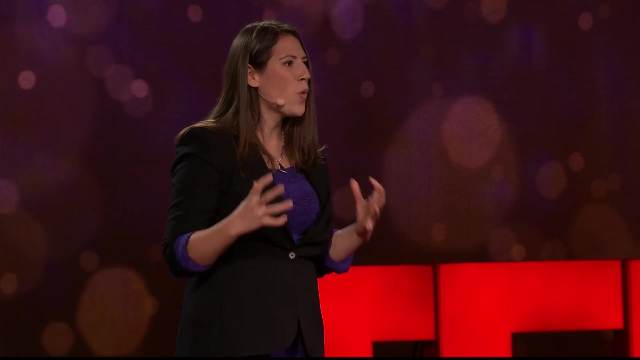 Mohegan stories, our language and culture is the integration of ideologies instead of boxes and binaries. In Mohegan, you don't separate art from politics, from education, from the earth, from you, from me, from our community. Everything is woven together because there are no hard lines. 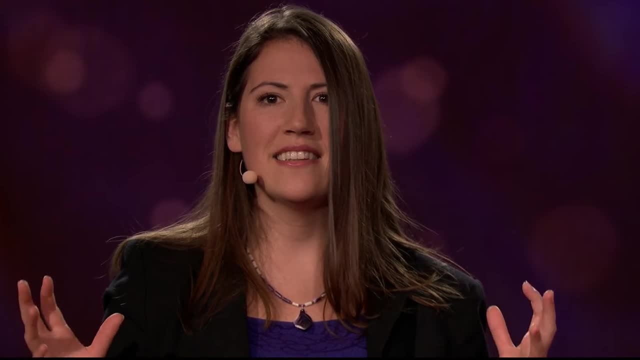 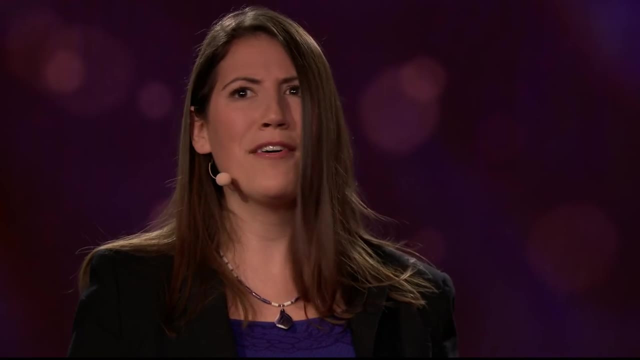 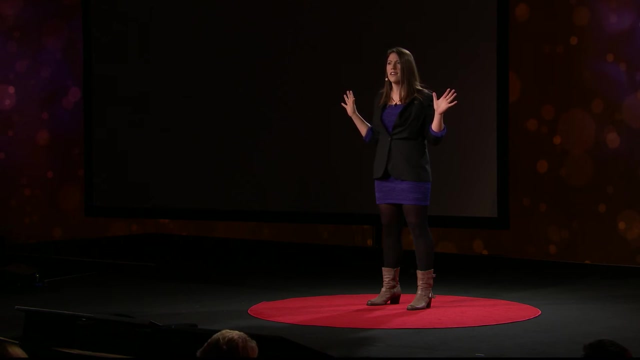 breaking up our universe. Ideas lean on each other like people, So I started to wonder what happened. How did we lose this community connection? Who decided that that person at the front of the room was suddenly more important or magically all-knowing, instead of what they are a part of? 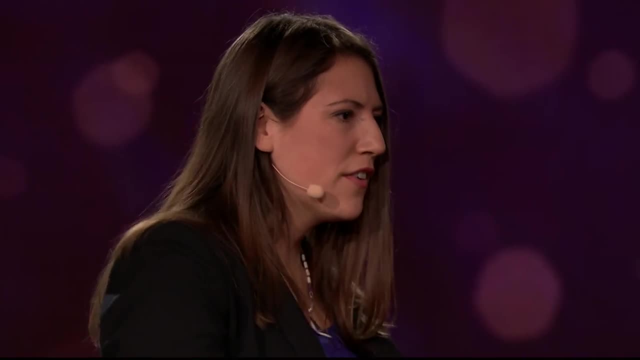 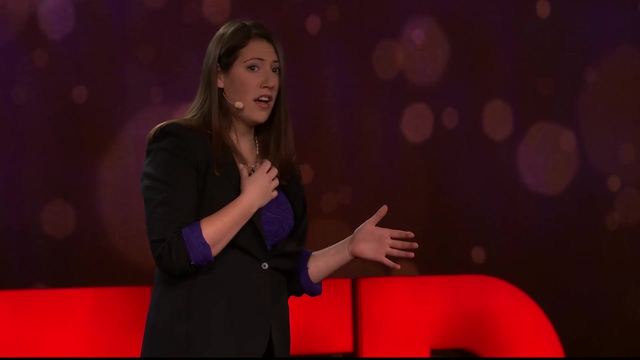 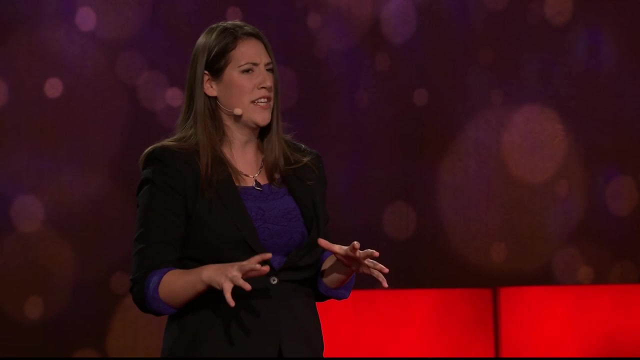 the group. What happens if we look for connections instead of divides? Lead from a place of listening, from a place of love. As someone who directs both in and out of the native community, I became aware of a divide where the theater industry's language seemed to be: 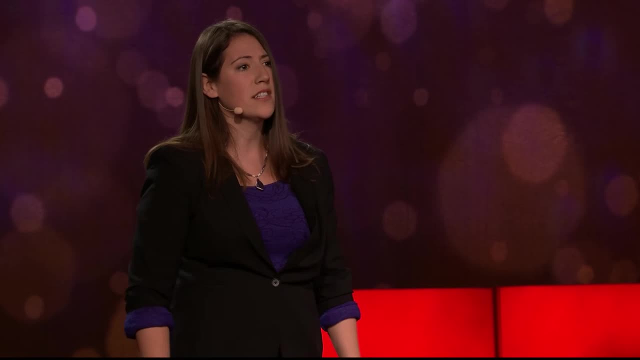 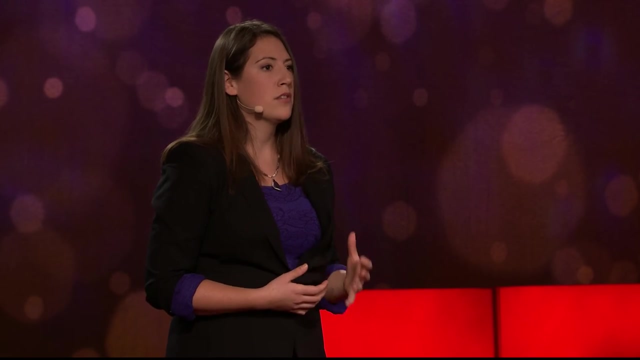 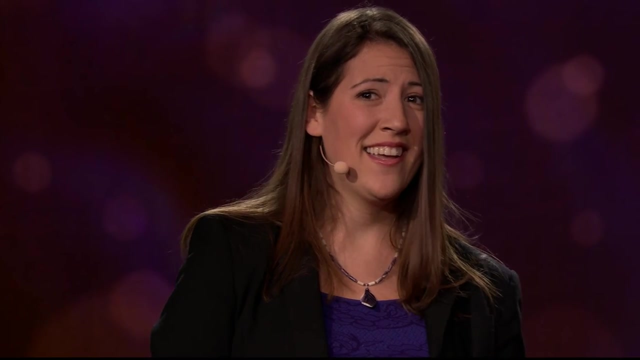 poisoning what I believed was important about the process of telling stories, of building worlds on stage. Frustrated, I went and I spoke to one of my friends and mentors, playwright William Yellow Robe, about it, one of the fathers of contemporary native theater. He told me to really 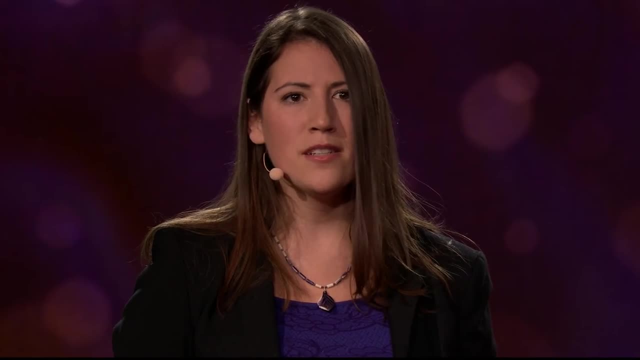 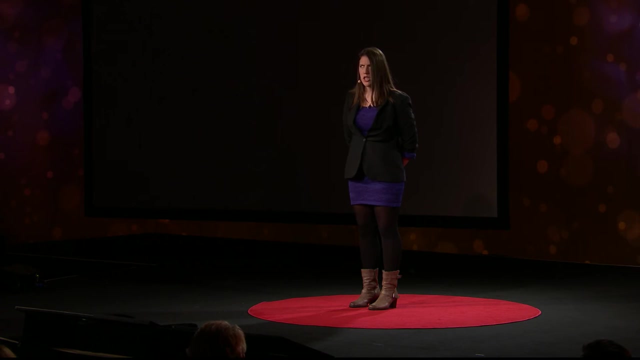 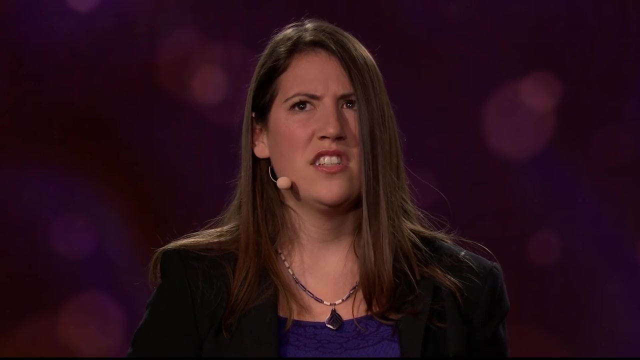 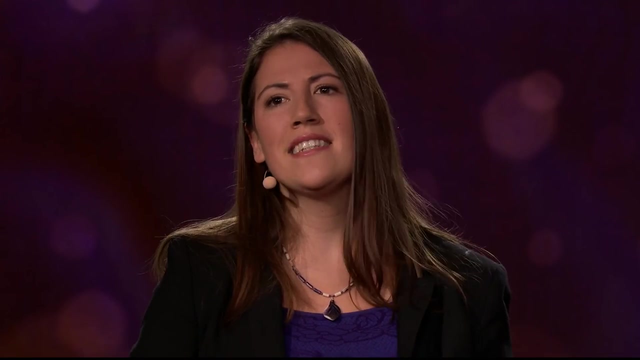 have a strong native theater movement, we needed to be using the words in our own languages for what we were doing. Director- The word director is not particularly elegant, imaginative, passionate. When I hear it, I think of someone directing traffic, barking orders, aggression, and I realized I don't want that job. So I went and I asked: